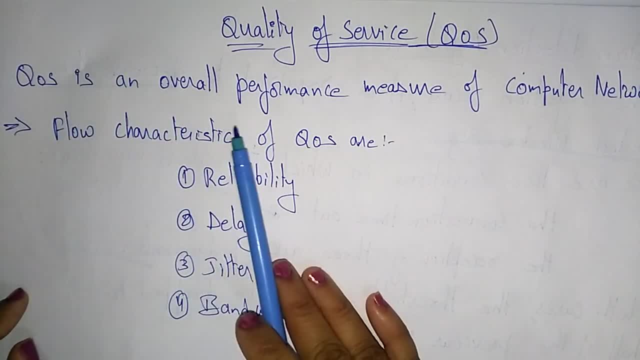 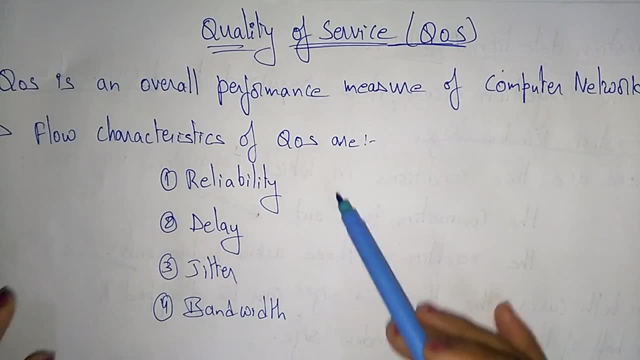 QOS, The quality of service, is an overall performance measure of a computer network. So there are some flow characteristics of quality of services there. that is the reliability, delay, jitter and the bandwidth. Now let's see. what is this? reliability first. 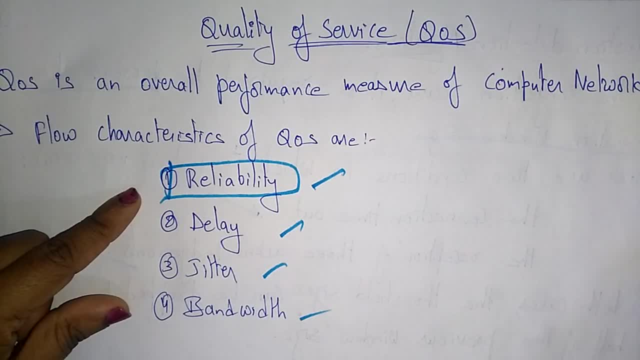 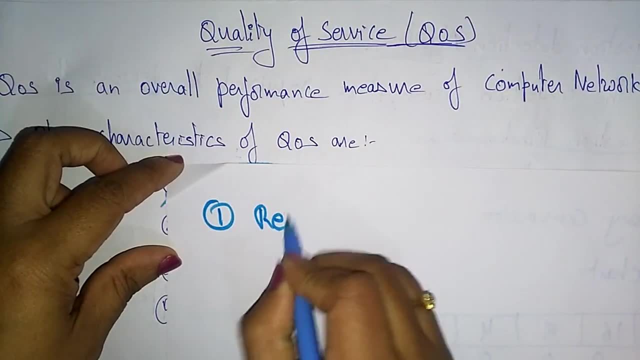 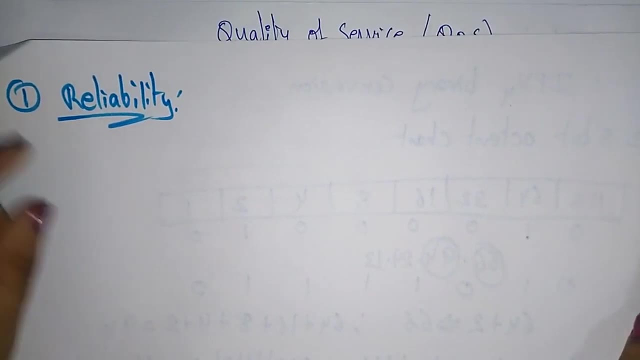 So reliability. let me take the paper. I will explain that actually the reliability is a first one is reliability, The first flow characteristics of quality of service is reliability. So, if a, So if a packet get lost, let's think that if the packet get lost or acknowledgement is not received, 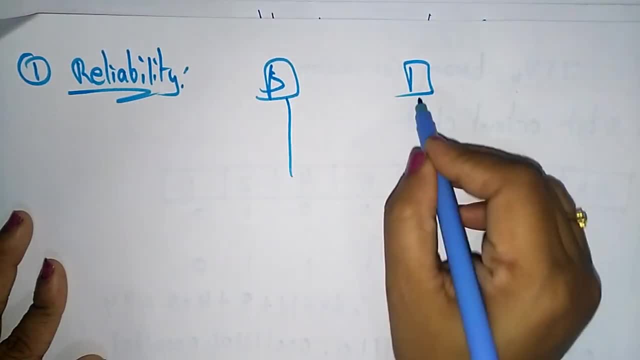 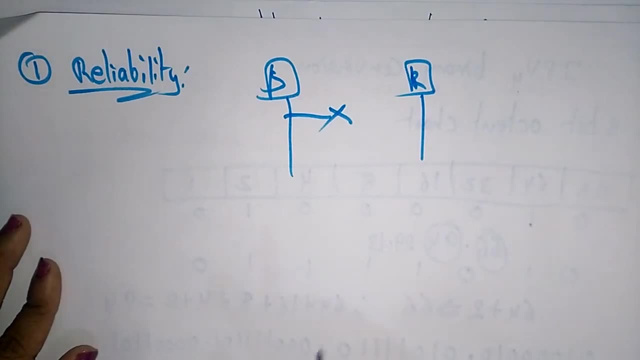 the sender is sending the message and the receiver is receiving the message. Suppose the packet is lost or it doesn't receive any acknowledgement, then what you will do? you again retransmit. Okay, again, the retransmission of data will be needed. So what happens here? 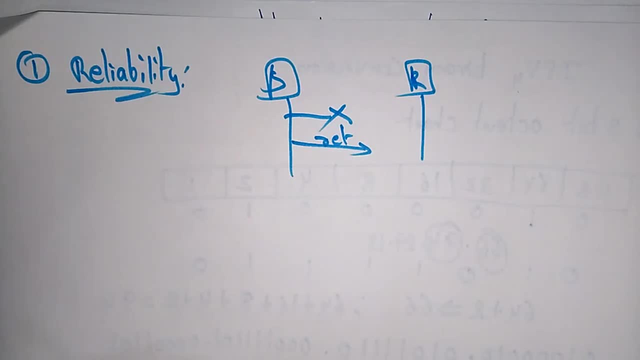 the reliability is decreasing. So whenever the retransmission is taking place, this decrease the reliability of the system. Okay, so if a packet gets lost or acknowledgement is not received, the retransmission of data will be needed. this decreases the advailability. Let me take one example, like email. 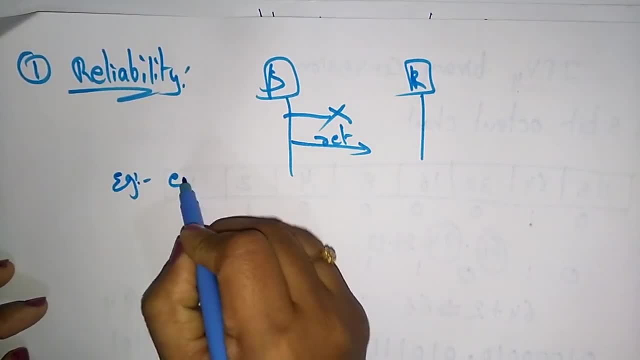 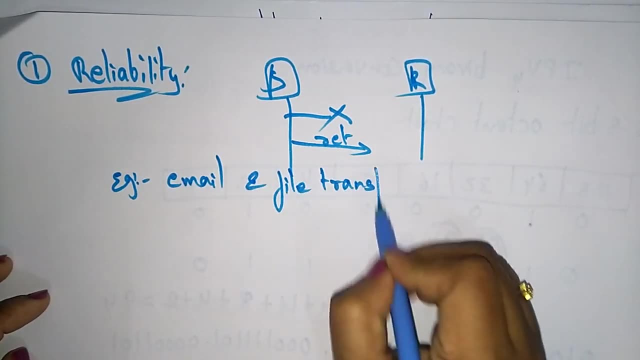 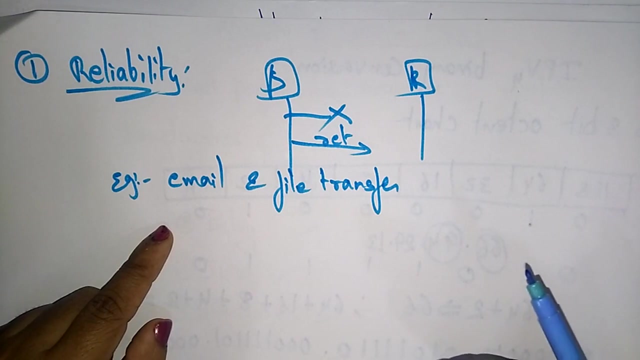 The examples of the reliability email and Fight transfer. So here the email draft. Let me see that again. Let me check that: Announcement not received. whatever the email communication, the file transfer you are taking in those concepts, you need a real able transmission as compared to that of an 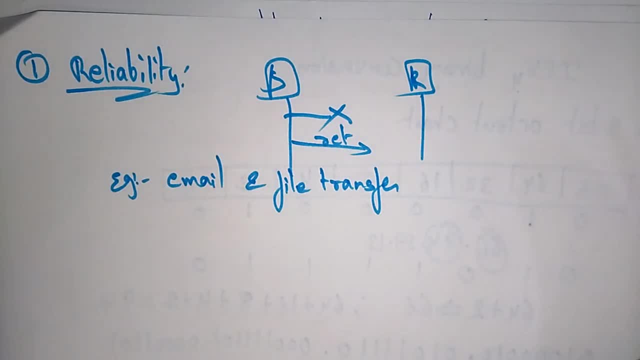 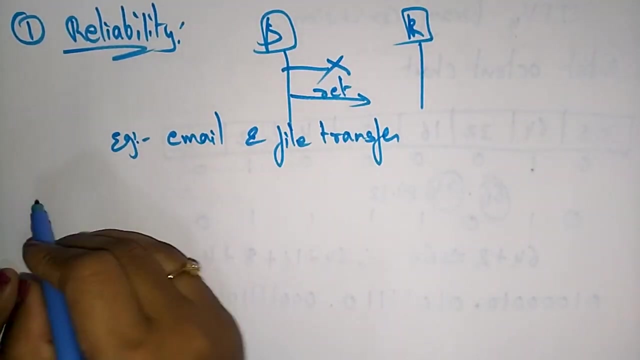 audio conferencing. so rather than and compared to the audio conferencing here in the email and the file transfer, you need a real, able connection whenever you are sending the data. you have to receive the acknowledgement within some times. okay, so that is the first quality of service. that is a real ability. next, 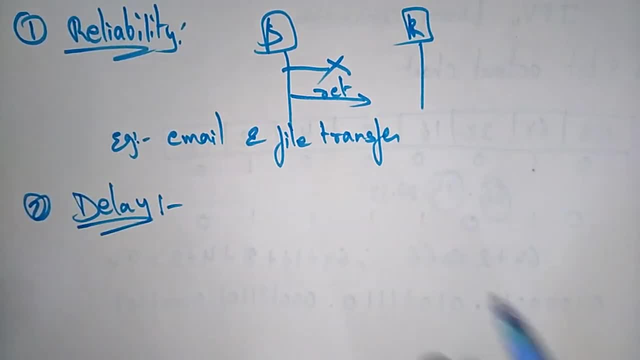 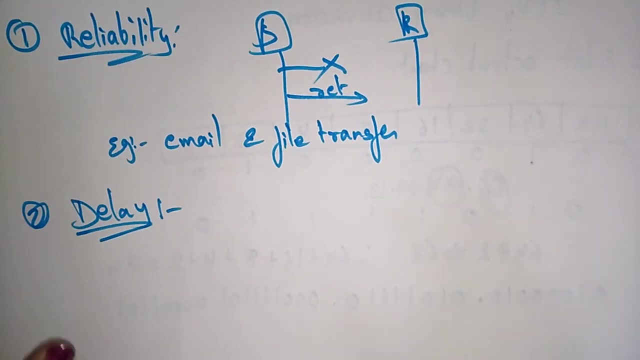 is delay. we know what is a delay. delay is doing something slowly. okay, it's getting the information slowly because of delay, some something is happening in between the source and destination. that is a delay. a delay of message from source to destination is a very important characteristics. let's take the 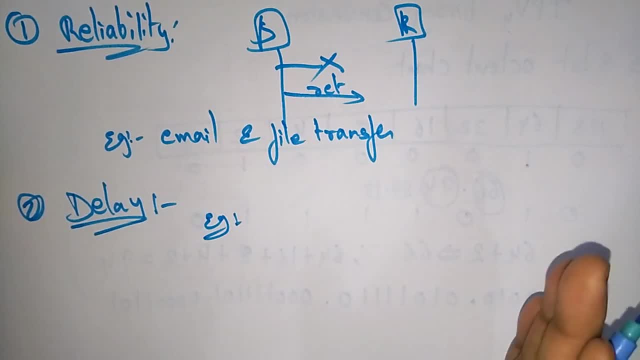 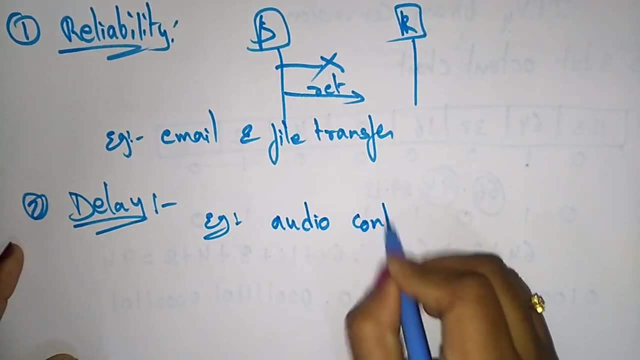 example here, a time delay. the time delay cannot be tolerated in audio conferencing. let us take audio conferencing as an example. so here in the audio conferencing, the time delay cannot be tolerated. why it is cannot be tolerated? because while you are communicating you need some delay should. 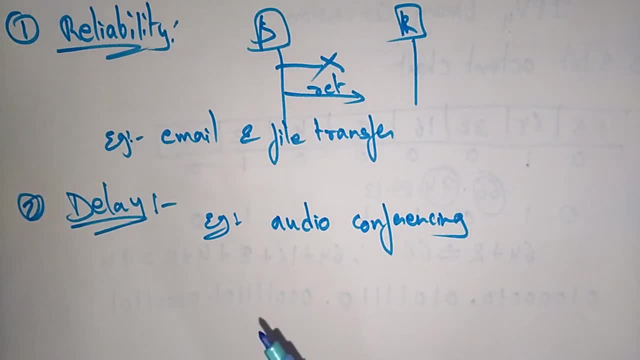 be there. it needs a minimum time delay, okay, so, while time delay in email has less important, okay, while I am talking to you, okay, if I communicating with you after after, after, after I am completing my word, you can able to talk with me. otherwise, if you, if you. 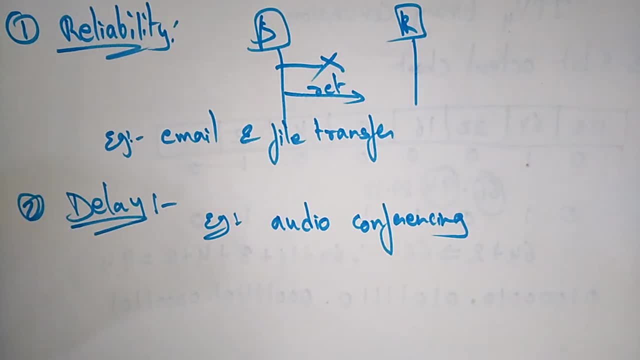 didn't receive my message clearly and you are going to respond to my question. if my question is not completed and you are responding to my question, means it's somewhat disturbance, is there? it is not toleratable, okay, the time delay cannot tolerate. in audio conferencing its needs minimum time delay, whereas in email. 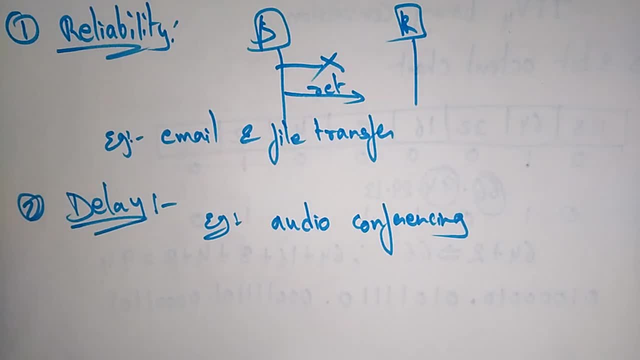 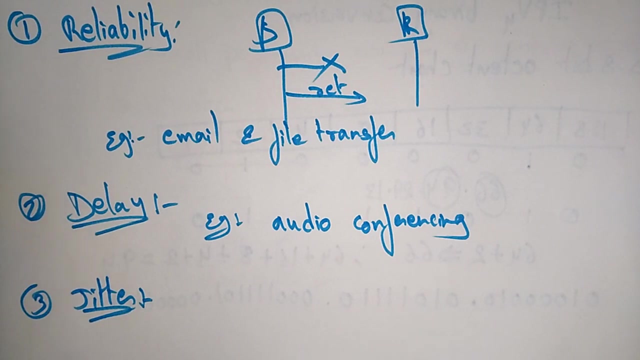 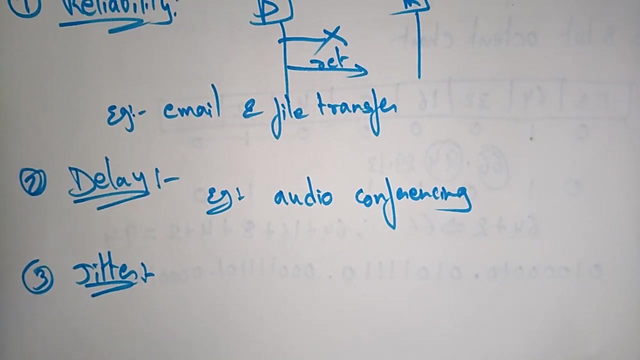 conferencing email, if you take it, has a less important on time delay. so that is one of the quality of service flow characteristics. and the next is a jitter- jitter. what is this jitter? it is a variation in packet delay. a jitter is nothing but a variation in packet delay if difference between delays is larger. 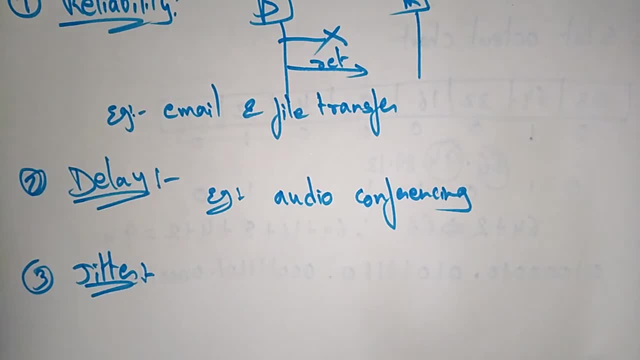 than it is a high jitter. if the difference between delays is smaller than it, is a low jitter. high delays, is there large jitter and the small delay is the less jitter. let me explain with one example. suppose three packets or sent at a time. three packets or sent at a time? okay, so first let's take 0, 1, 2. 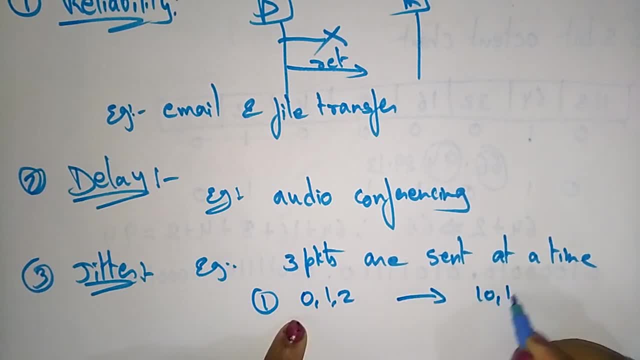 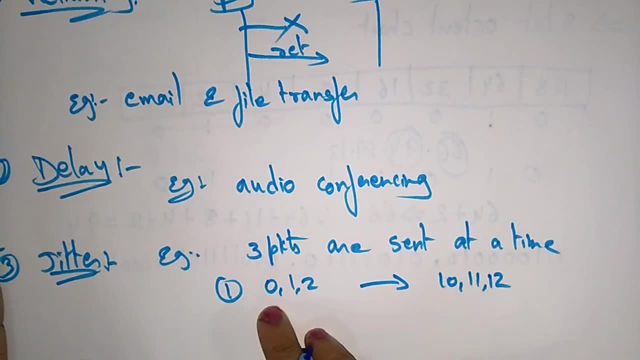 these packets are received at 10, 11, 12. okay, so 0, 1, 2 at the time, 0, 1, 2, 3 packets or at time, 0, 1, 2 and the receiver side. it reaches the packets 10, 11, 12. so did you.